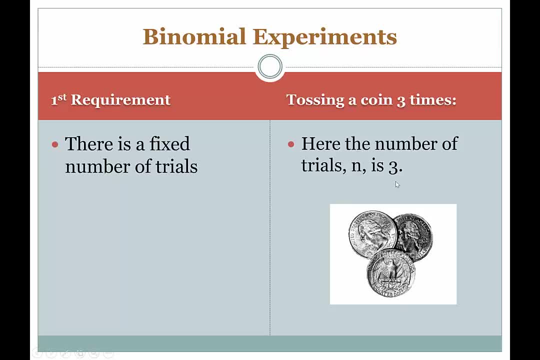 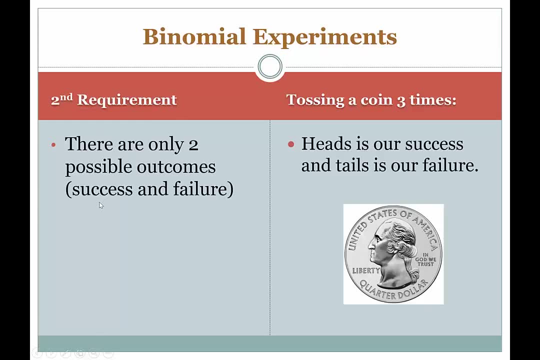 tossing the coin three times. So here the number N is three, right, So we have three tosses, So we have a fixed number of trials. The second requirement is there are only two possible outcomes for each trial: success and failure. Well, yeah, if we're looking to see how many heads turn up, we can label. 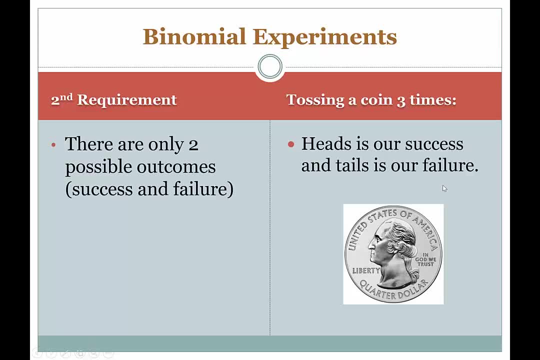 heads as a success, right And tails become the failure. And there's only two possible outcomes then: heads or tails, or success and failure. All right, the third requirement is that the trials are independent from each other. Sure, one coin toss should not influence the other coin tosses, right? So we know coin tosses. 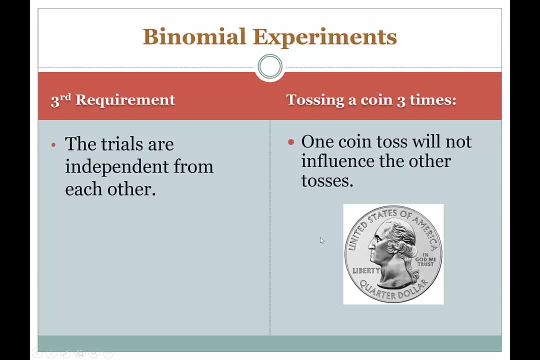 are independent of each other. So we can say that it meets that requirement. All right, the fourth requirement: the probability of success should remain constant for each trial. So whatever chance there is that the coin turns up heads, that should remain the same. 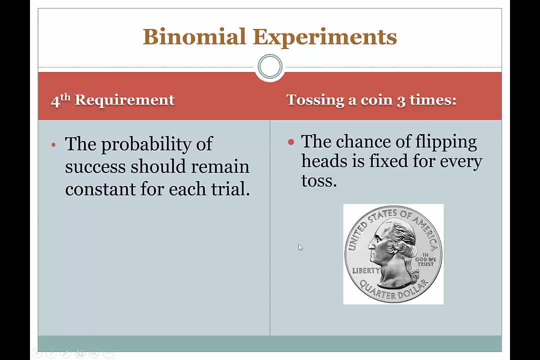 throughout the tossing right. So in other words, if it's a fair coin, the head should come up one half of the time. And again it would be the same for the first toss and the last toss and the second toss right. In each case there'd be a one half chance. 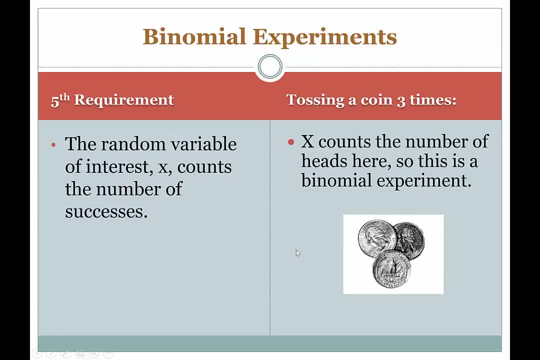 that the coin turns up heads, So it meets the fourth requirement. And then finally, the random variable of interest, x, counts the number of successes. We said in the beginning of the problem that x would count the number of heads here. So, and that means in this case we can say this is a binomial experiment, because heads were. 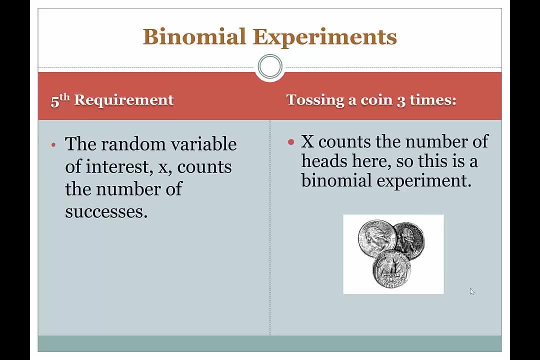 defined as our success. So x counts the number of successes, And that's it. we can consider tossing a coin three times and counting the number of heads that turns up- a binomial experiment, By the way, of course. if you counted the number of tails that turned up, that's also. 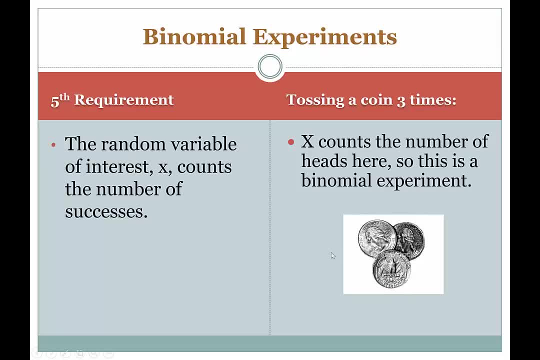 a binomial experiment. you just have to pick one or the other right, Okay, And then from there. the next thing we want to talk about briefly is the binomial probability formula. So if I want to know the probability of success, I'm going to have to do a little bit of a 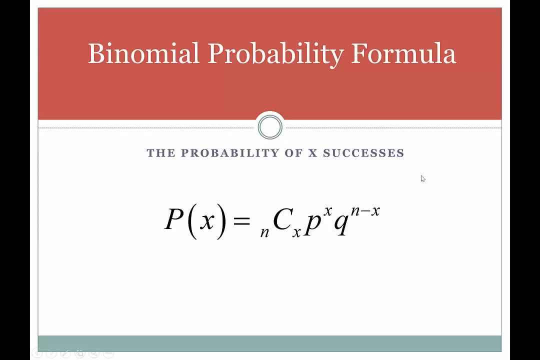 test. So if I want to know the probability of a specific amount of successes out of n trials, this probability formula will give me that answer right. So it's the probability that we have x successes, for example, in that last problem. what's the probability? 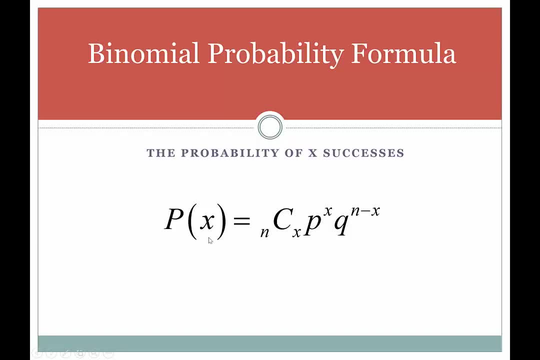 that we end up with two heads on the coin. Well, x would be two, then two successes. we'd have three flips, So the little n here would be three. This is a combination, So it'd be out of three flips. choose two of them to be heads or two to be successes, right? 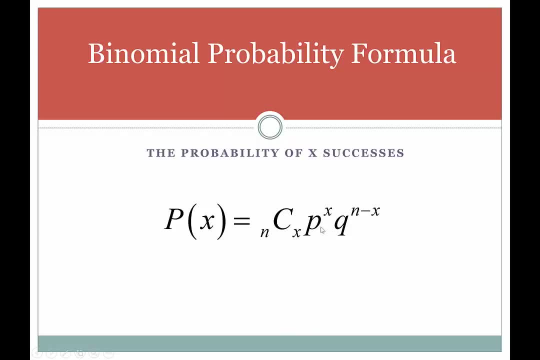 So three choose two, The probability. here P is going to represent the probability of success, right? So P stands for probability, In this case it's the probability that we end up with a heads, because that's our success in the experiment. And if the probability of heads would be one half, if 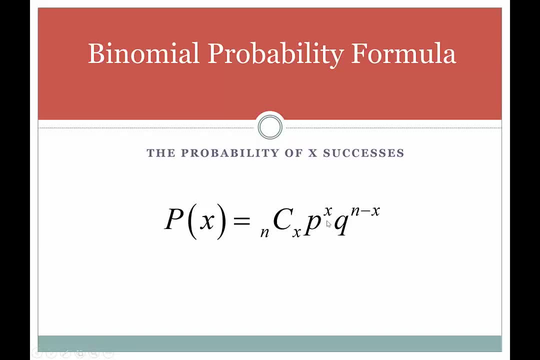 the coin was fair, so we'd have one half and we'd raise it to the second power. Why do the second power? because we're looking for two heads or two successes. heads is our success. So one half raised to the second power because we'll have two heads. And then what? this expression? 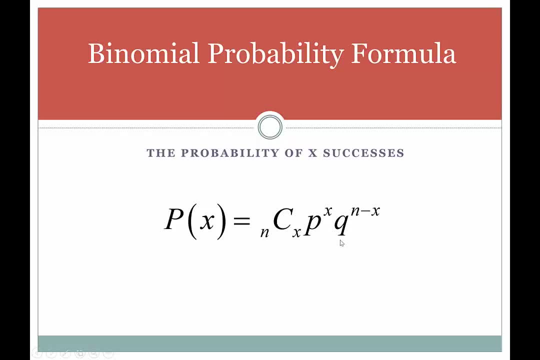 is is all the leftovers. And what we mean by that is we're going to say, hey, what's the chance that we fail to get ahead? What's the chance that a failure occurs? In this case, a failure is a tail. What's the chance of a tail? It's also one half right, So P. 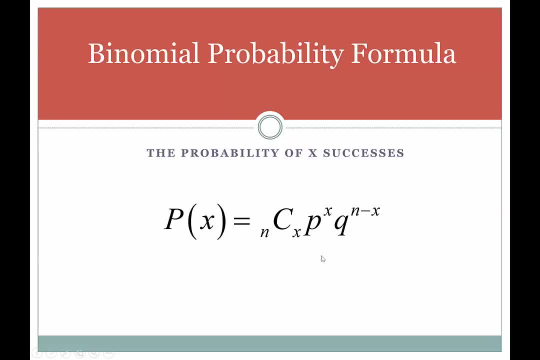 and Q must add up to one. Or in other words, if you want to find Q and you know P, you can do one minus P and that will give you Q right. So it's the leftover probability from 100%. There's a 50% chance you end up with the heads. There's a 50% chance you end. 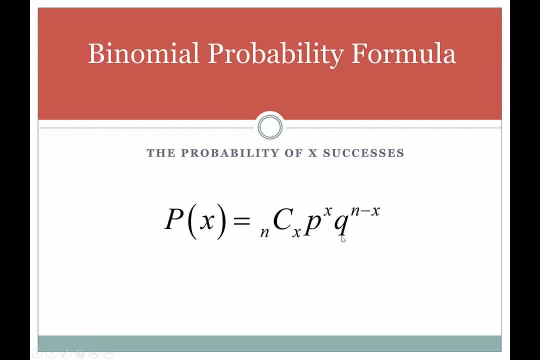 up with tails, because 50 plus 50 add up to 100, right, If there had been a 10% chance here, this would have to be 90, because 10 and 90 add to 100.. If it was 20,, this would have to be 80.. If this was 30, this would have to be. 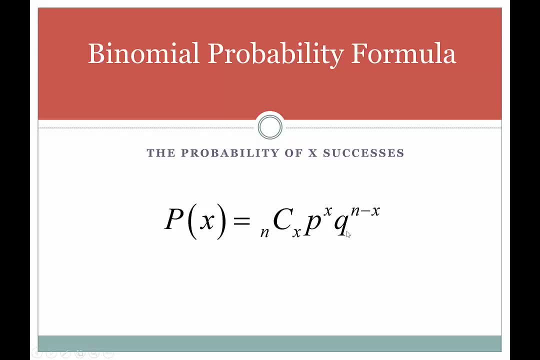 70. If this was 60,, this would have to be 40, right, So on and so forth. And then N minus X is also a leftover of sorts, right, Because if we're saying we're going to have X successes out of N trials, right, In this case we're tossing the coin three times and 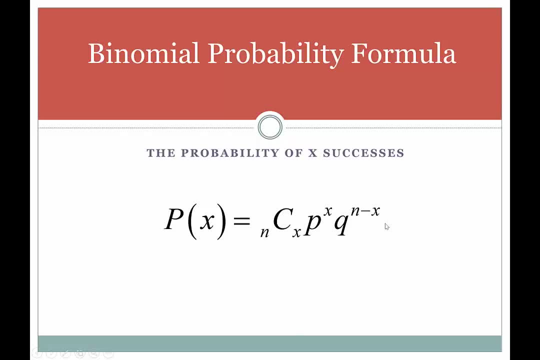 we're going to have two successes, Then N minus X must be three minus two, Leaving you with one. In other words, we're simply saying: hey, if we're going to have two heads, then we should have one tail out of three tosses, right? Because if it didn't, 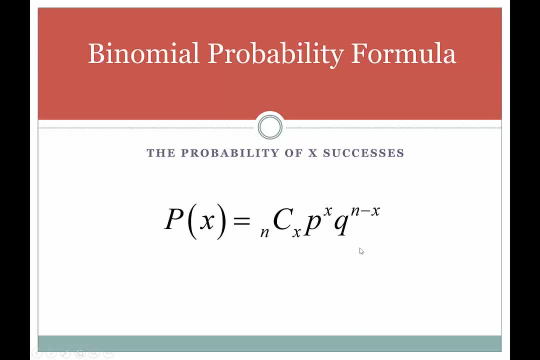 turn up heads. what did it turn up? The failure in this case tails. So this number has to add to this number to get N back right. So if two trials are successful, then one trial must be a failure. if you have three trials, total right. So that's basically the idea.